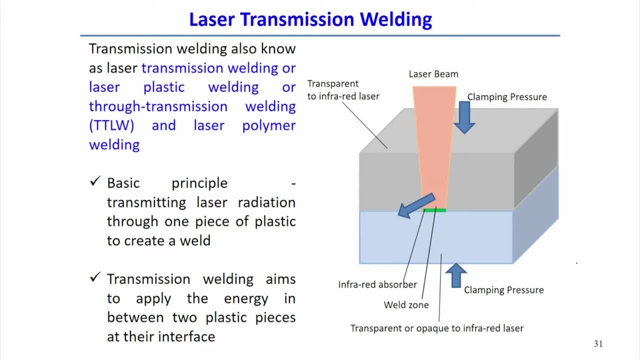 it will melt the surrounding area And by applying the some clamping pressure or applying some forces for a specific time period, then welding of this joining can occurs after cooling down of this molten steel. So this is as simple if this is a laser. 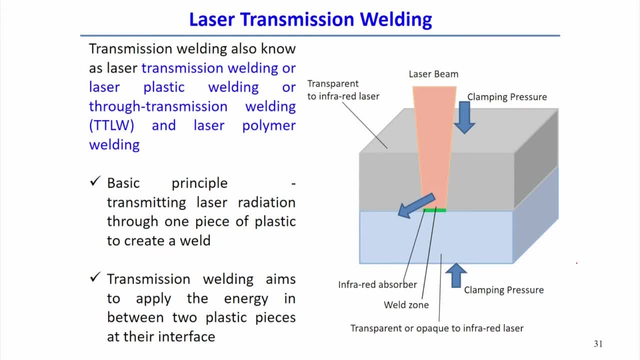 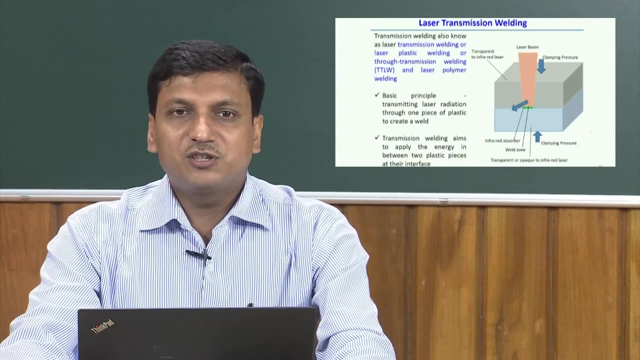 transmission welding, but sometimes this transmission welding is also known as plastic welding, laser plastic welding or through transmission welding and sometimes laser polymer welding. So basically this welding process has been developed in specific application for the polymeric material. So basic principle is: 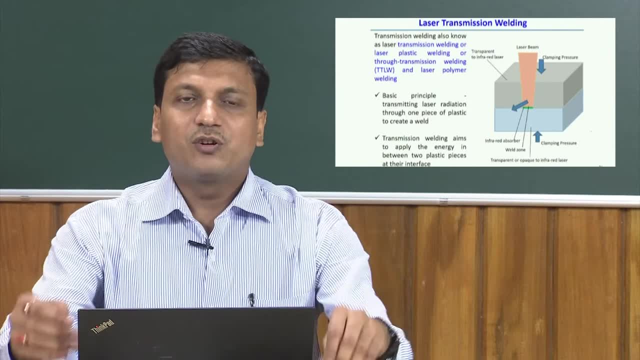 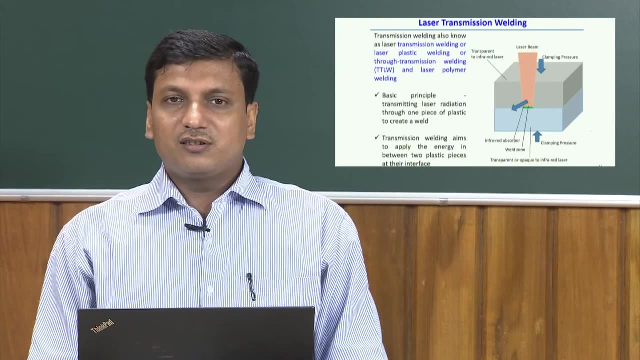 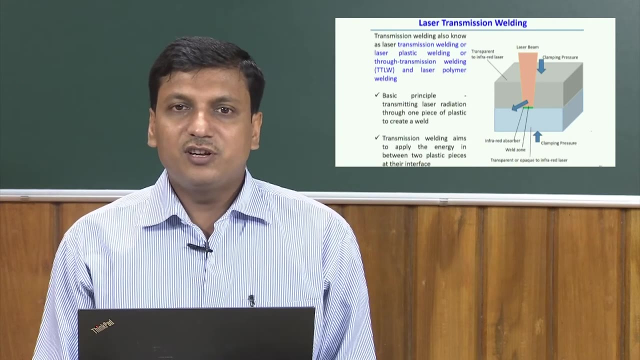 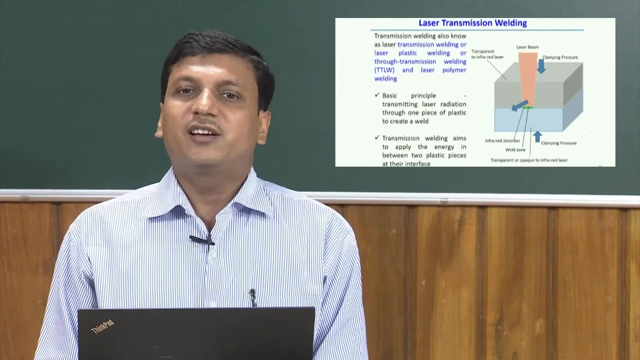 that transmitting laser radiation through one piece of plastic materials to create a weld. So once the transmission come just through one layer, then some energy in between these two layers have to be released such that at the interface there may be joining of between these two components can be done. 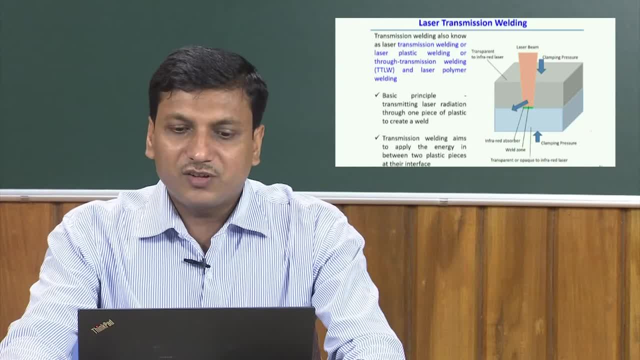 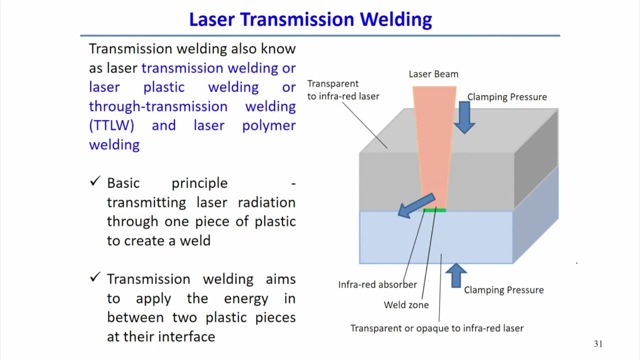 So here, if you see the figure, that transparent laser, but that transparent, that laser, transparent through this material, that is, the. it depends upon the wavelength of this specific laser, which laser is used here, and it is a infrared or near infrared laser mostly. transmittance happens for a different types of the polymeric materials. 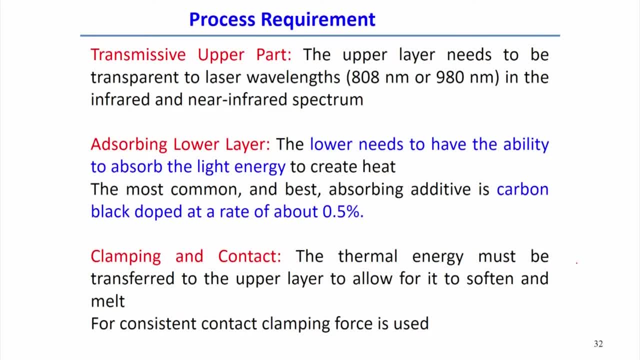 So if you look into further the process requirement for the laser transmission welding is that first the transmitting upper part, the upper layer or upper components, needs to be transparent to laser wavelength. So actually the transparent transparency of the laser light depends on the wavelength of the laser specifically used for the welding process. 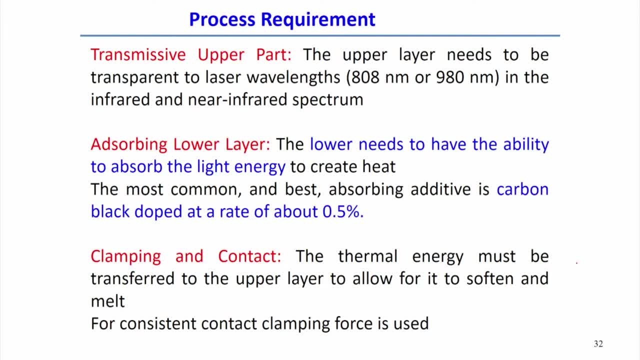 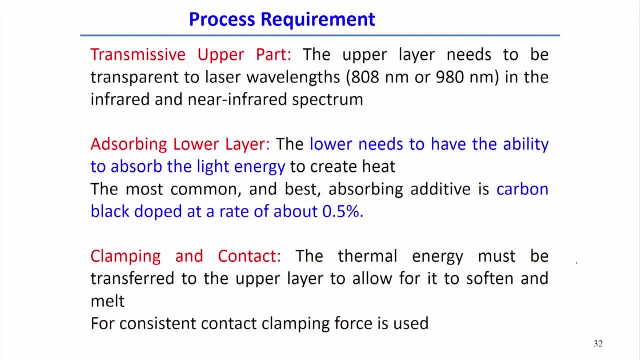 or near infrared pextrum, So in that range if we use the laser, and that laser is. 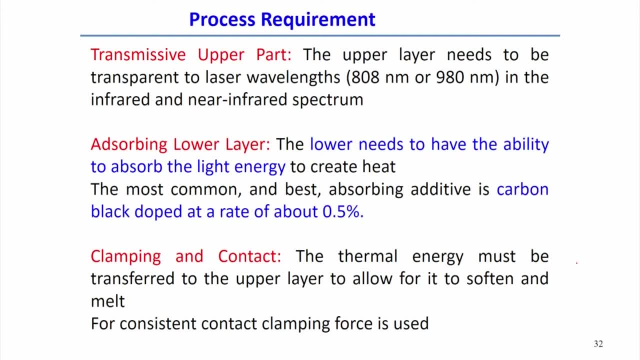 basically applicable for the laser transmission welding. So once transmission upper part. next component is with the absorbing lower layer. So absorbing lower layer, so that we have to choose the lower layer component in such way that the that layer will be able to absorbs the laser energy, laser light energy to 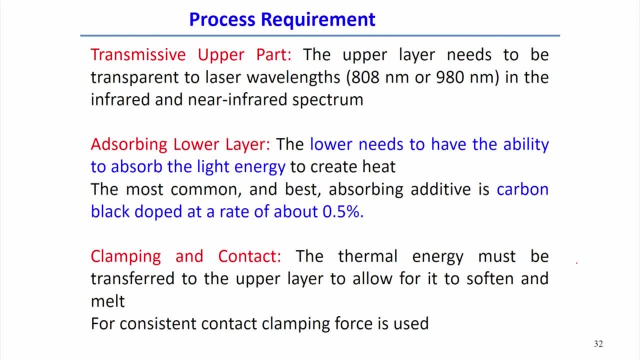 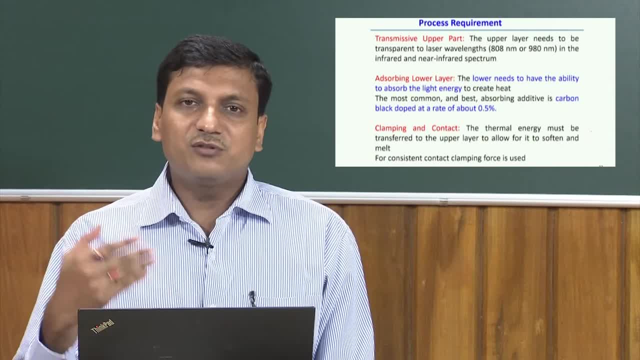 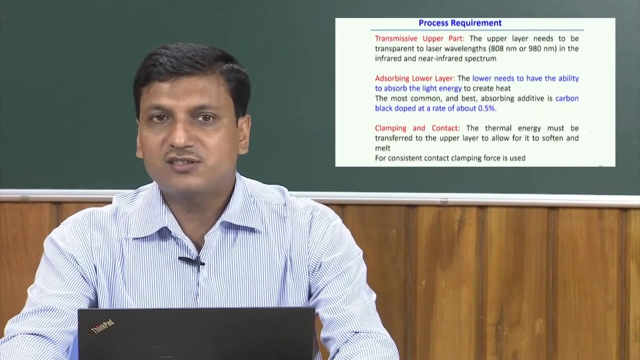 generate the some amount of the heat at the interface. So sometimes if both are both polymeric material are transmissive in nature with the specific wavelength of the laser used. So in that case sometimes some additive, absorbing additive such as carbon block, carbon black, doped at a rate of around 0.5 percent. that 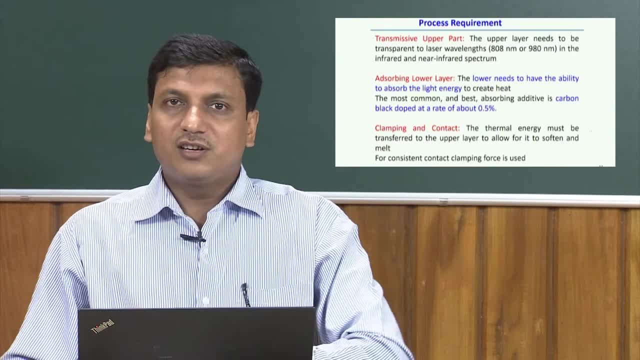 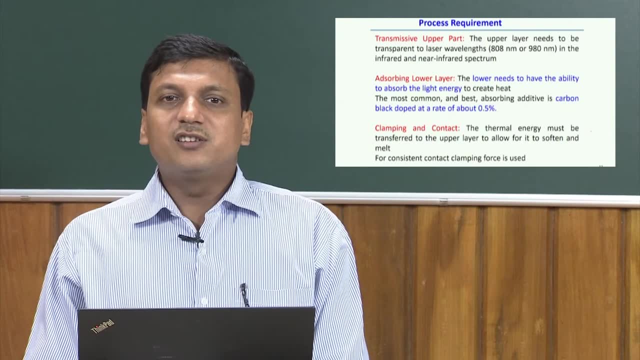 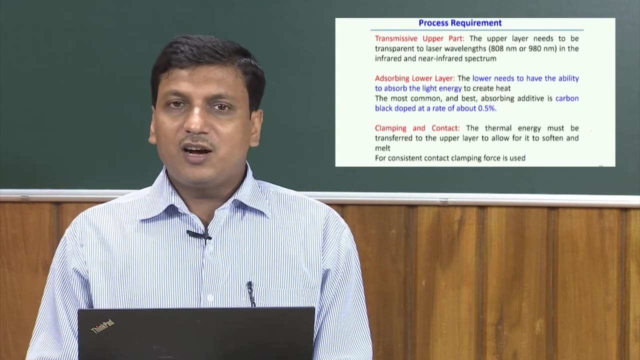 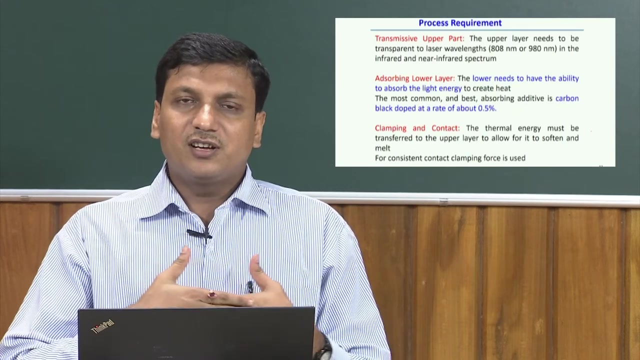 means that carbon black can be used at the interface layer. So that interface layer, that carbon black actually acts, basically absorbs the laser energy and creates some. So once the transmissive layer and then absorbing layer and after this the third process requirement here is that glumping and contact. So contact should be- is that it is a very 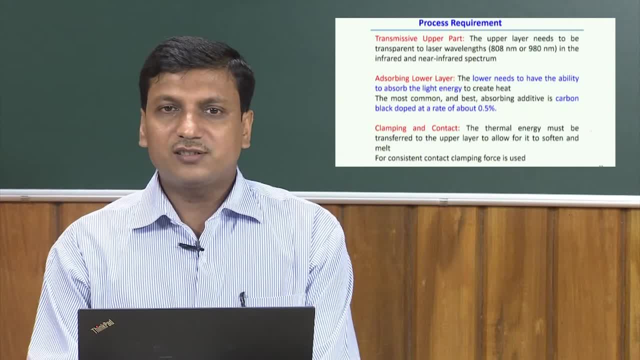 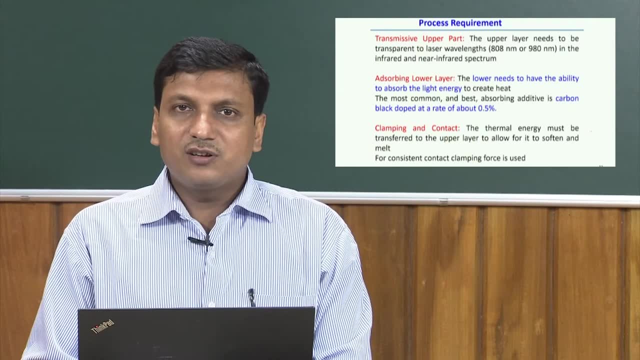 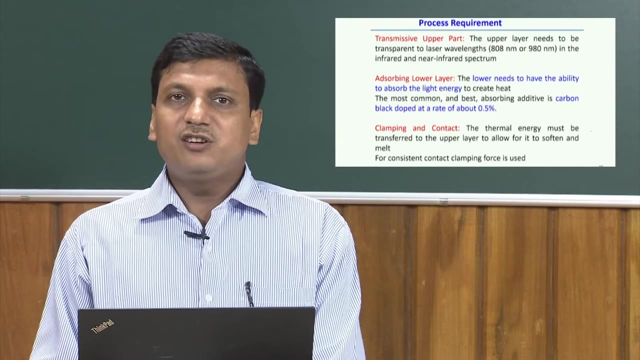 the gap between these two components should be very low, such that once the thermal energy is released on the at the interface, That means either in the absorbing lower layer- that means lower component- or on the interface. So then gradually heat will be conducted a to the upper layer, So that amount of energy will be also at the same. 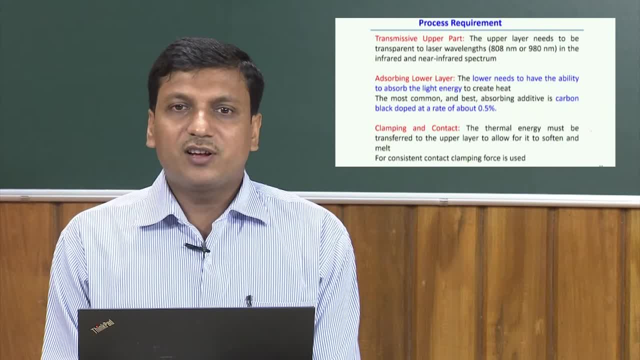 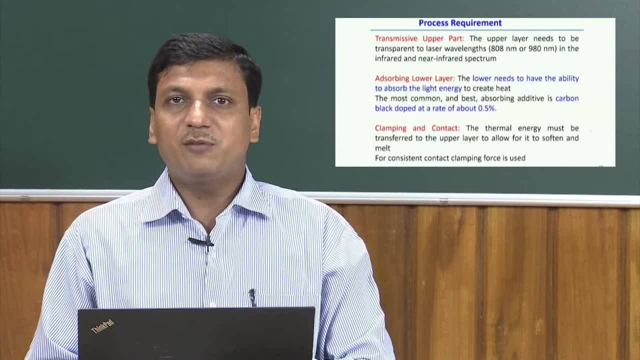 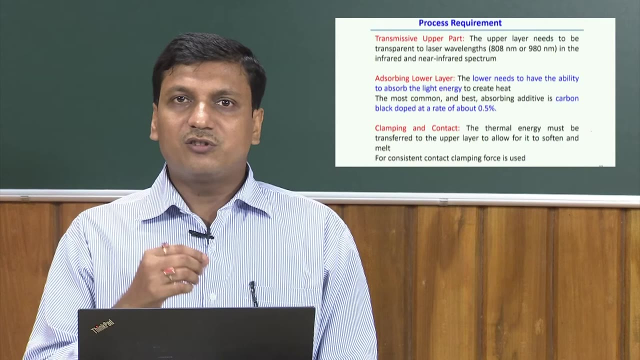 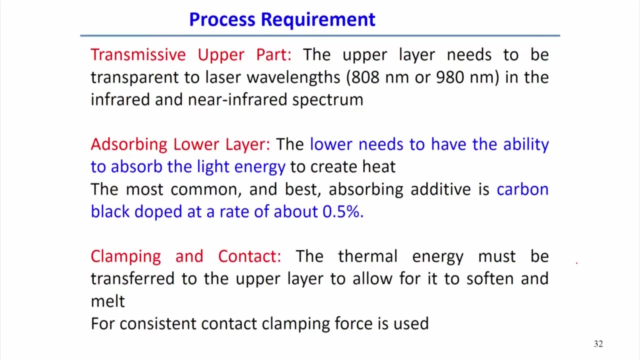 time will be able to melt the upper layer. Then only to make as a consistent contact between these two component, there is a requirement of the application of the some amount of the pressure between these two. So after cooling down this component, the strong well bit or can be formed for this polymeric material through laser transmission welding. 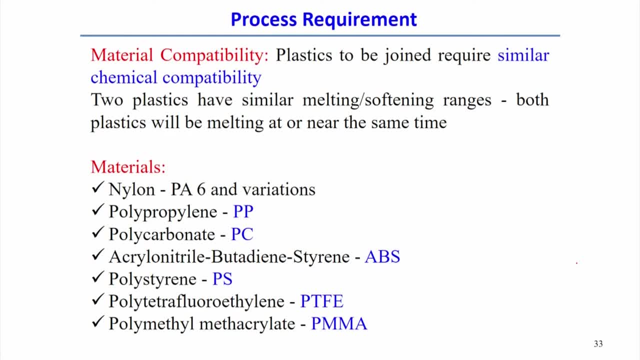 So material compatibility. you can see most of the plastics to be joined require similar chemical compatibility. that means two components have to be chosen. in such way, almost similar compatibility should exist. So at the same time, the two materials having the melting and softening ranges for both the plastic should be at the same time, or may not be that? 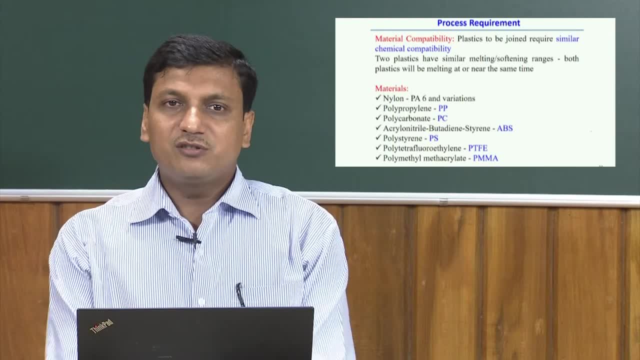 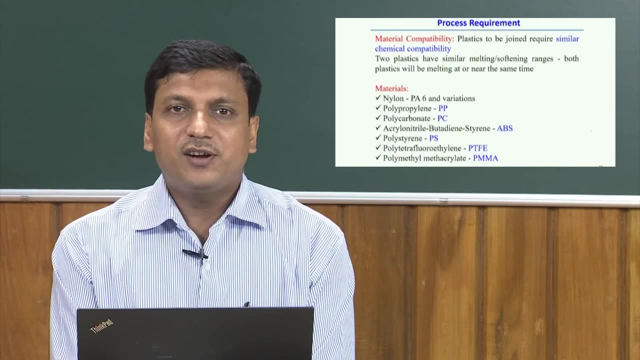 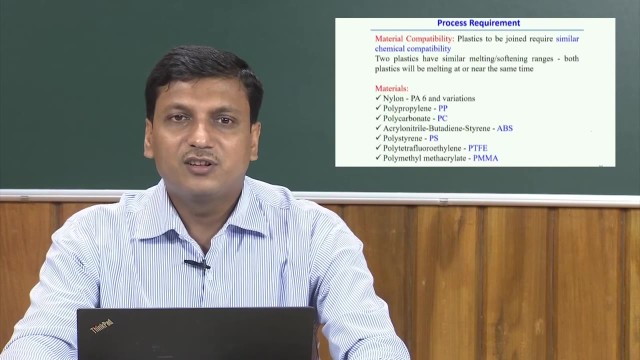 means there may not be much difference in the melting point between these two components, which is supposed to join by laser transmission welding. So if we see the typical materials applied or weld or joined by this welding process, it is that: is that nylon different, that P A 6 and that different variants can be joined. 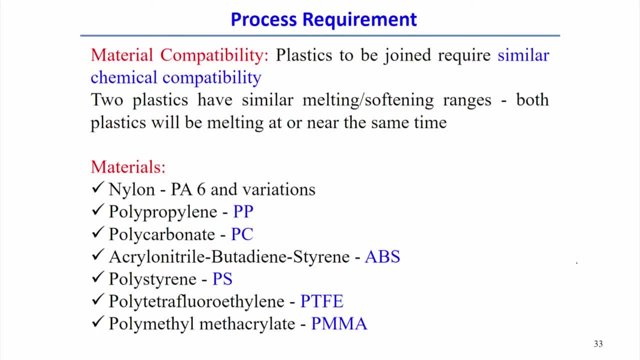 then P P, then P C, A, B, S, polystyrene- this is the short form of this- different polymers That can be joined using the laser transmission welding, the P T, F, E, and that P, M, M, A. all this type of materials can be joined by using the laser transmission welding. But if you look 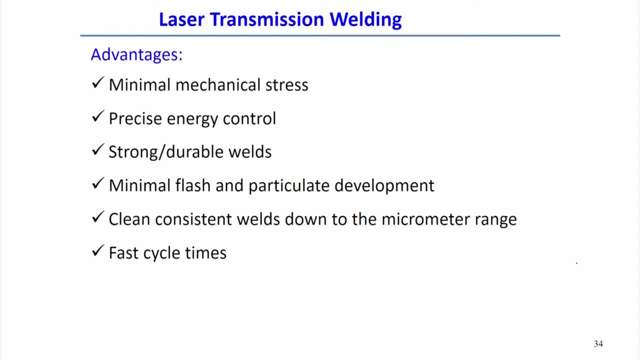 into that advantage. that means with respect to the other processes here or other welding processes. So here you can find out that there may be some minimal mechanical stress, so mechanical stress will be very less. There is a difference in the expense. thermal expansion coefficients, or may be, is the very 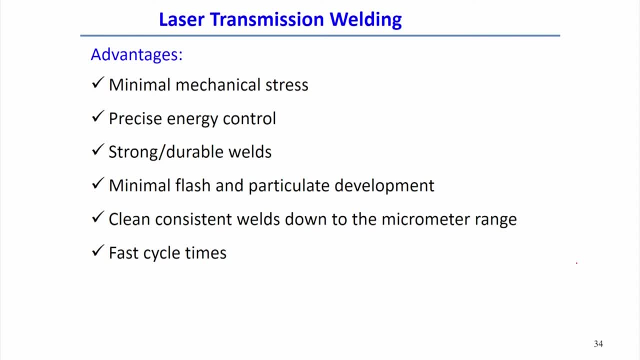 less in between these two, So there is a less chance to generate large amount of the mechanical stress. precise energy control: since we use the laser as a source, then we can very precisely focus on a specified space in the. therefore it is possible to control the amount. 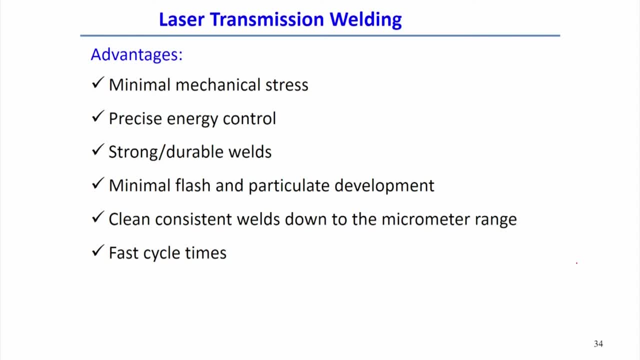 of the energy released at the interface, Then very strong and durable welds can also be done using this process by this process and, of course, minimum flash and particular development, which is very negligible in this process, and this process is very clean process also And the weld joined. that means heat. 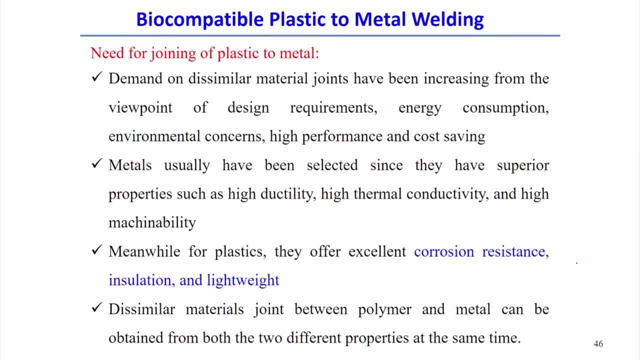 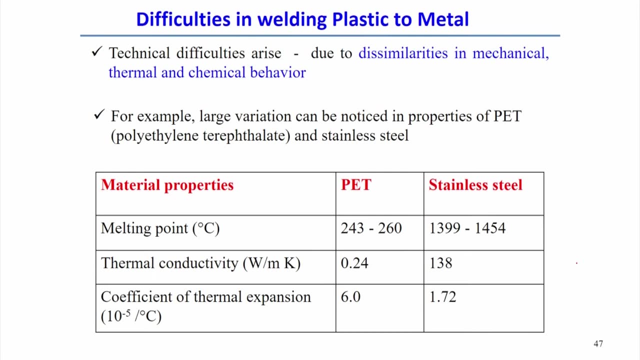 brings a huge difference in the properties. So therefore joining or welding of these two components, metals to plastic, has a huge difficulties because their properties are completely different. And not only that, they are different, not only the mechanical properties, even thermal and chemical behavior are also different. So therefore we can take an example also. 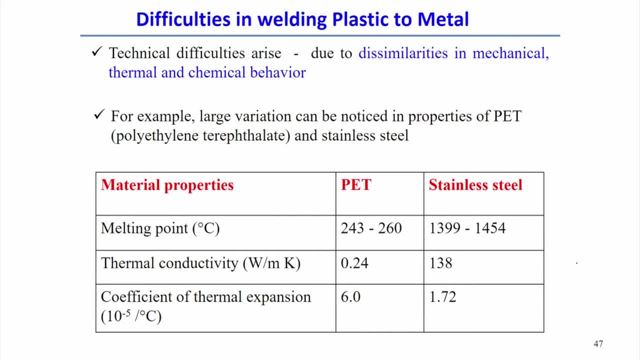 if we see that there is a two material, PET and stainless steel, and we suppose we want to join these two. one is the plastic, another is the metal, stainless steel. So here we can see the. there is a huge difference in the melting point temperature. one is the 243. 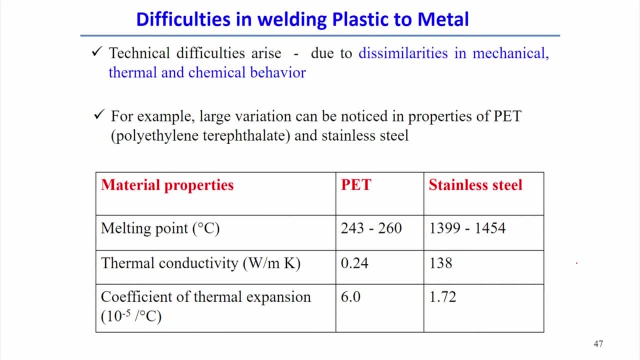 to 260 degree centigrade, another is the around 40 degree centigrade. So there is a huge difference in melting point, thermal conductivity also having huge difference. one is 0.24, one is the 138, other is the thermal expansion of the coefficients. 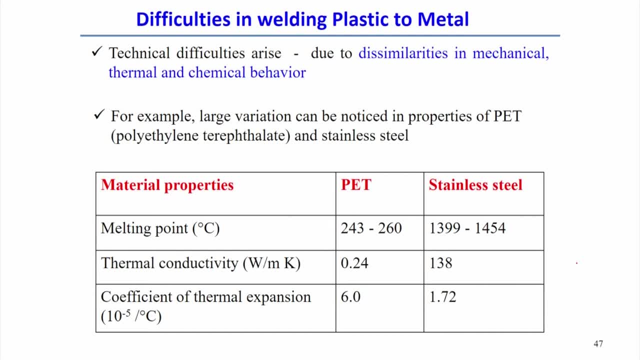 here we can see that one is: the thermal coefficient of the thermal expansion is 6 into 10 to the power minus 5. another case is 1.72.. So although there is a huge difference in the mechanical properties, But as I mentioned in particular it is, it is the 20submission aspect. 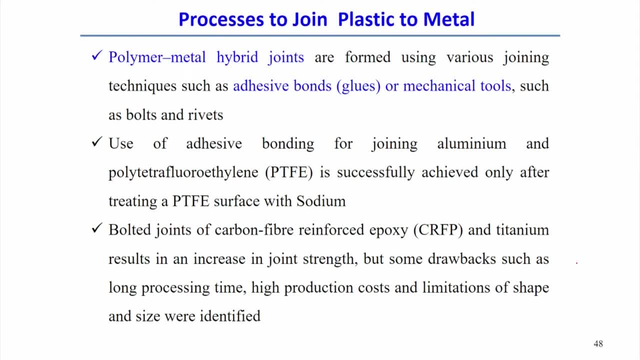 So therefore it brings. it is a very difficult to join between these two materials, but there are several methodologies also developed for joining the plastic two metals. One is the. this polymer metal. hybrid joints are found using the various joining techniques. simply use some adhesive bonds, simply using some glue or some mechanical tools. That is the 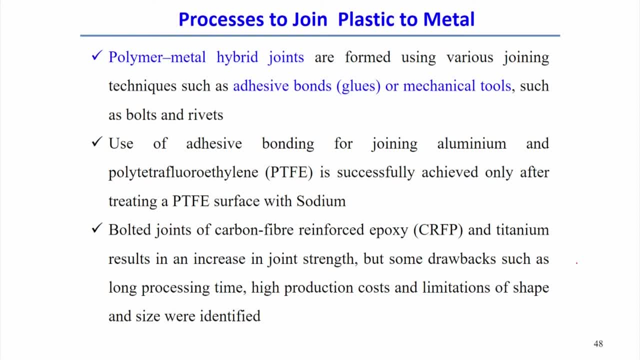 most convenient way to join between these two components. But use of additive bonding aluminum and PTFE we successfully achieved, but only after treating the very good surface treatment with the with sodium, that we observed the using the adhesive between the joining between aluminum and PTFE. So therefore, surface preparation is one. 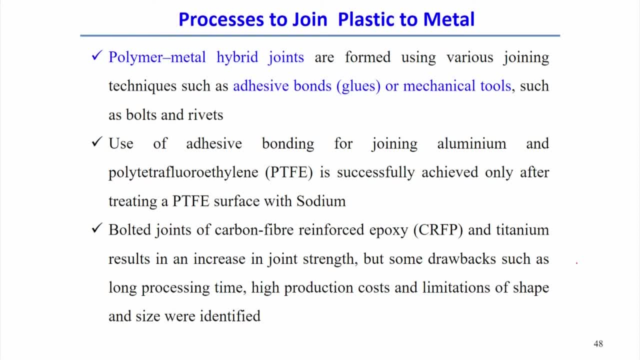 extra requirement in this case, otherwise bolted joint, some using some mechanical instrument, so simply bolted joints of the carbon fiber, reinforced epoxy, C, R, F, P and the titanium, that also having results in the increased joint strength. But definitely there have been some drawbacks, such as processing time is low processing. 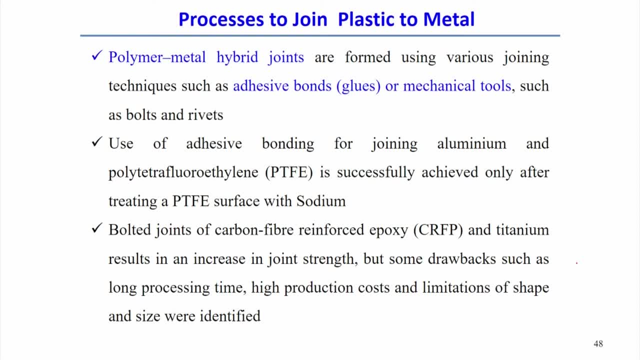 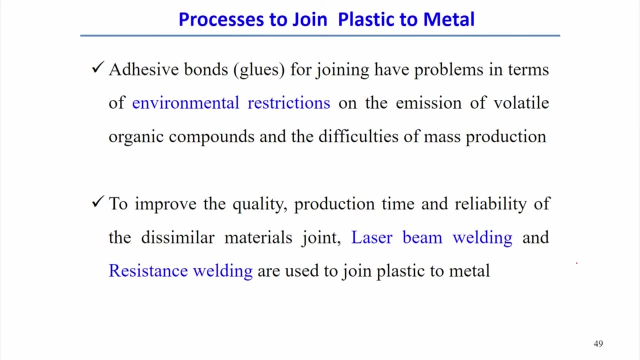 time. high production, cost limitation of the shape and size. that the main obstacle, using some means of the mechanical joining of these two components. But difficulty is that adhesive bonds, although we can use, or glue, we can use more easily for joining these two components, but problem is that it is a environment restriction is there on the emission. 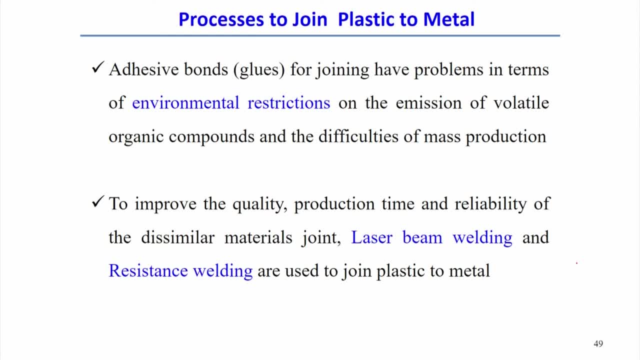 of the volatile organic components And at the same time there is a difficulties of the mass production using this adhesives or glues, and of course there is a some life span of this So glue, so in that sense it is limited. other way, the to improve the quality. 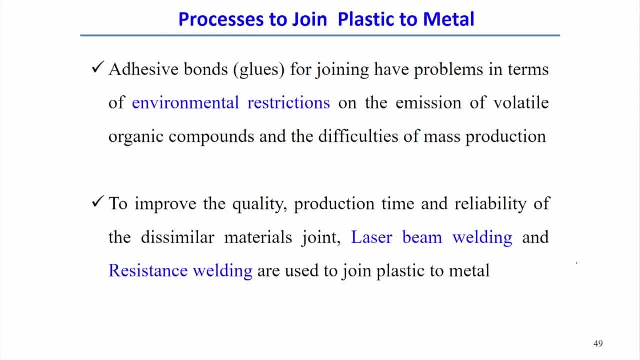 production time, because that is rate of the production reliability of the dissimilar material combination. in this case can be used the laser beam welding and the resistance welding. these are the two, mainly two, welding processes can be used for the joining of the plastic to metal. So, of course, if you look into the resistance, 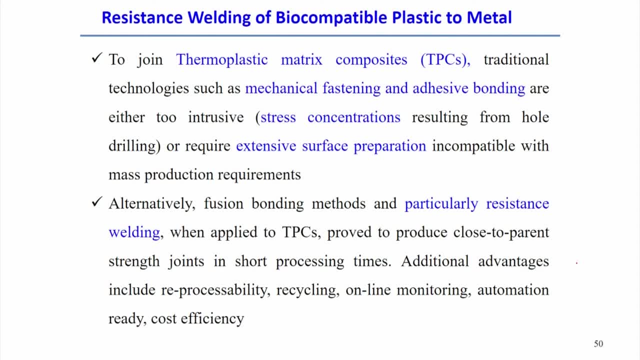 that TPC, that is, the polymeric material and joining process, such mechanical fastening and adhesives. So we can use it. but point is that here if we use the mechanical processing we can find out the stress concentration due to the hole drilling. that is the one things and there 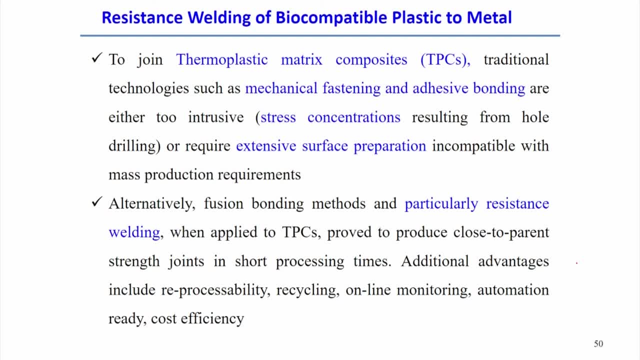 is a extensive surface preparation also required, So that actually incompatible for the mass production requirements. alternatively, that means in the to avoid this situation, the resistance welding can be used for joining the metal to plastic. So this, when we apply to TPC, prove to produce the close to parent strength. join because 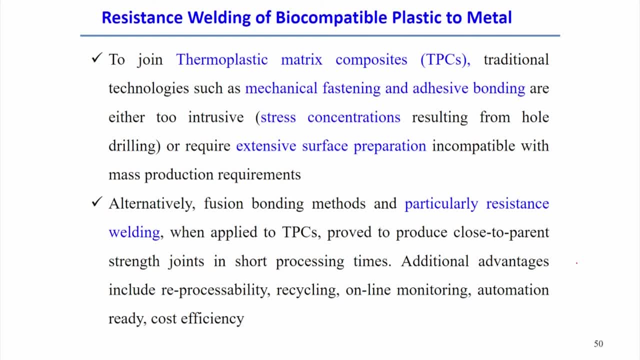 when you join these things in the short processing time using the resistance welding process we can find out. thus, joining strength is very much close to the parent metal may be in this among these two metals and the polymer, in which cases the strength of the base metal component is a low. if you can compare almost similar range of the weld joint strength can. 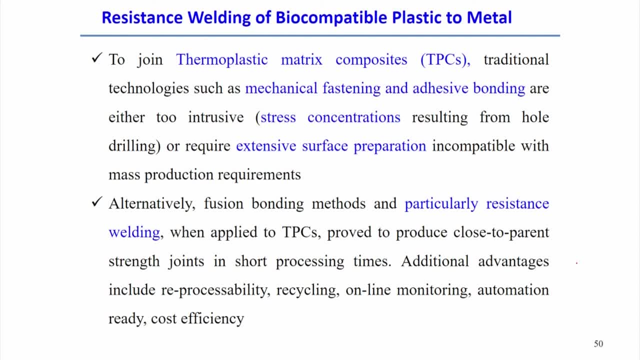 be achieved by joining, At the same time, additional advantage like reprocessibility, recycling, online monitoring, automation and cost efficiency. all in that aspect, the resistance welding of this combination metal to plastic is the better choice as compared to the other, using some adhesives or using 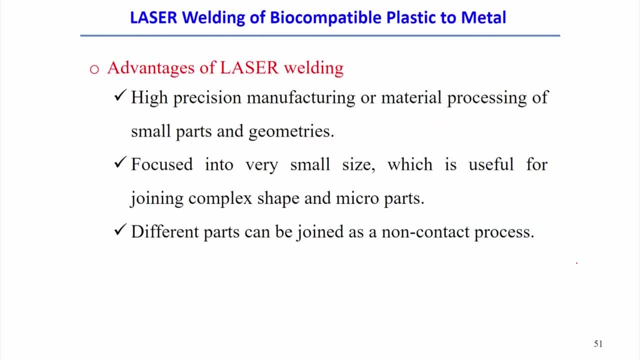 some mechanical joining Laser advantage of the laser welding is known to us also Because laser welding is known to us and has two advantages. So metal to plastic is that laser for lots and also like other metal to plastics are Because laser loading it is a high precision manufacturing for the material processing. 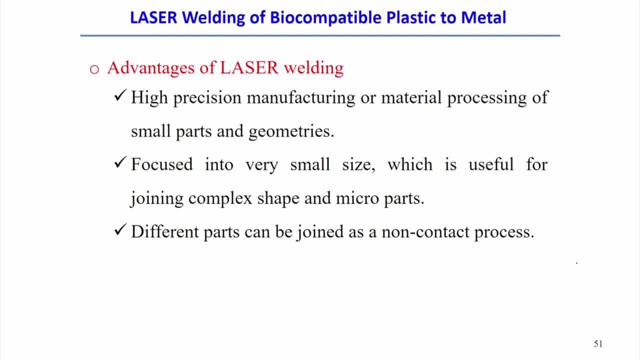 for the small parts and geometries, and laser can be focused into very small size which can be used for joining of the different components and even for the micro components can also be joined using some using laser. And other advantage is that laser is a non contact process, so therefore this is an added 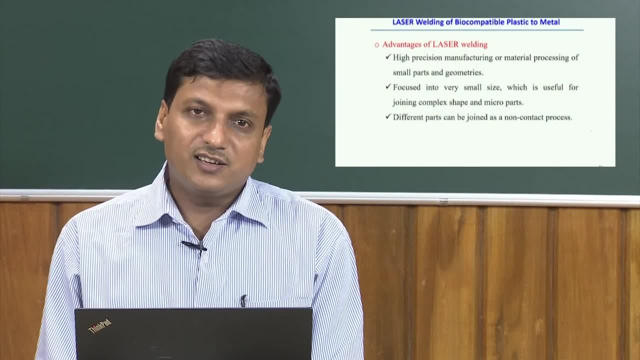 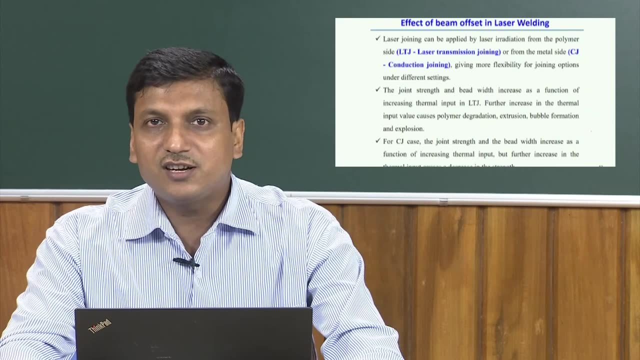 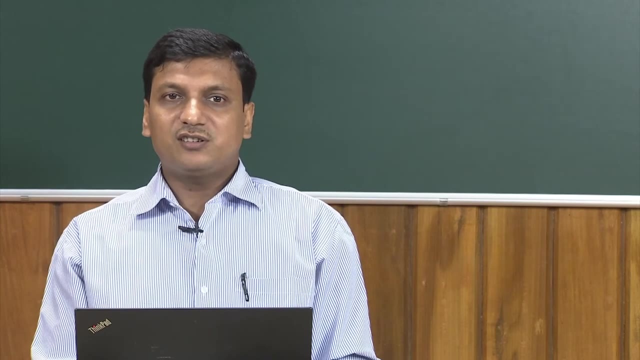 advantage of using the laser in specifically in case of the welding of the different materials. So therefore, apart from the resistance welding, laser transmission welding is the another option for the joining of the metal to plastic. So here we can see that already we have discussed about the laser transmission welding or laser transmission. 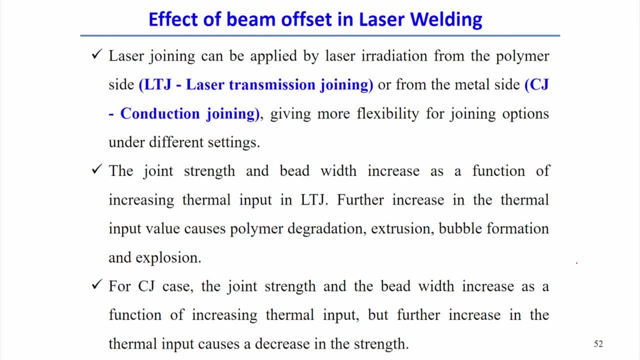 joining, in this case the polymeric materials. normally we can keep on the as a transparent material at the upper side and lower side. If we put the metallic material so, then therefore at the interface, so heat will be released on the metallic material and then we can join by the laser transmission welding. 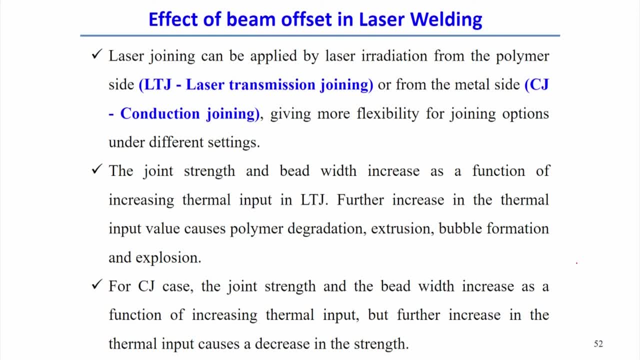 specifically easy to do that in joining between metal and the plastic. So it is observed that joint strength and the bead width that means increase as a function of the increasing the thermal input from the in the laser transmission joining. So therefore, if you increase the thermal 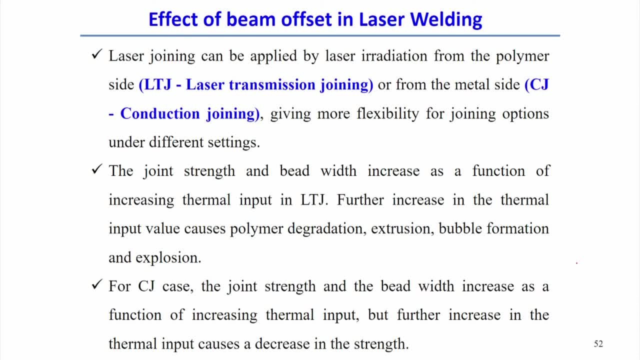 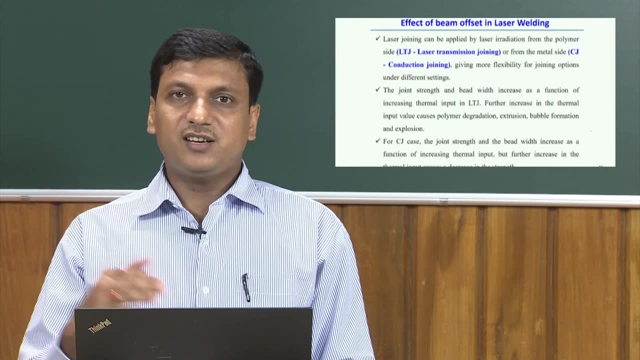 input. So then strength can be increased. but at the same time, if we increase too much, then there may be the degradation of the polymer and bubble formation. explosion. that can also happen. So we need a optimum amount of the energy such that the joint strength can be. 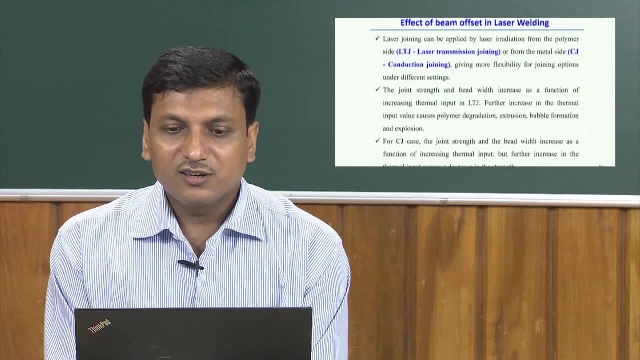 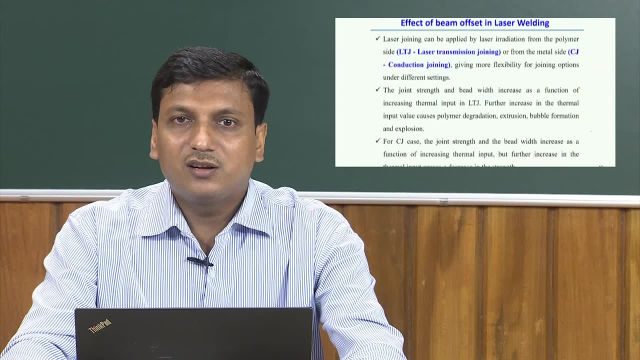 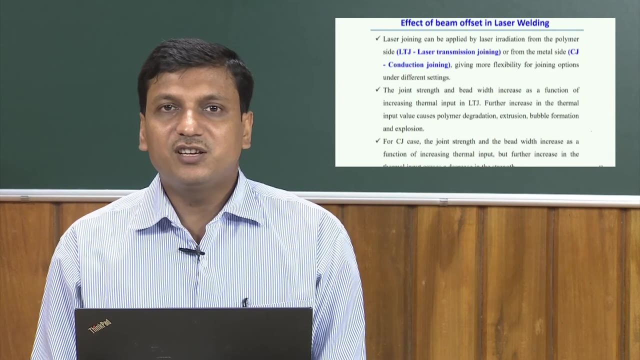 optimum between the polymer and the metal. But in one side it is called laser transmission welding, but in other side from the that is called the conduction welding, C j conduction welding. So in this case the joint strength and the bead width increases as a function of the increasing thermal input as well. but 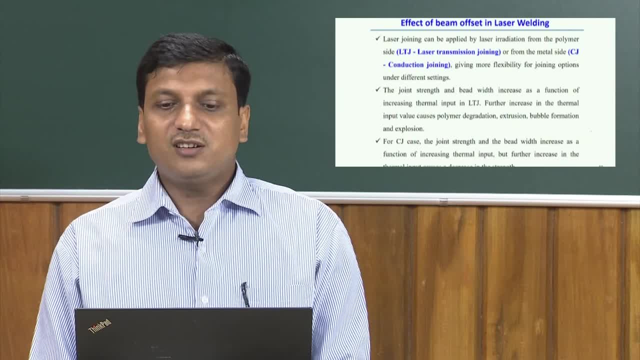 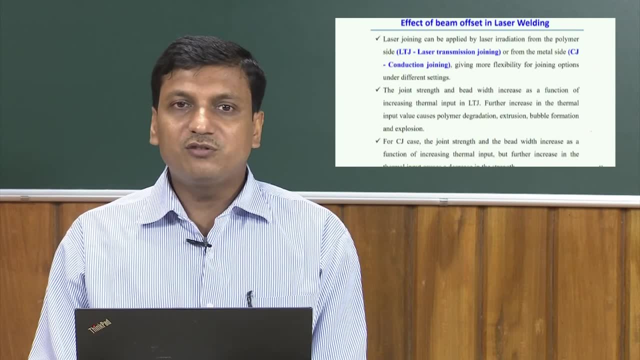 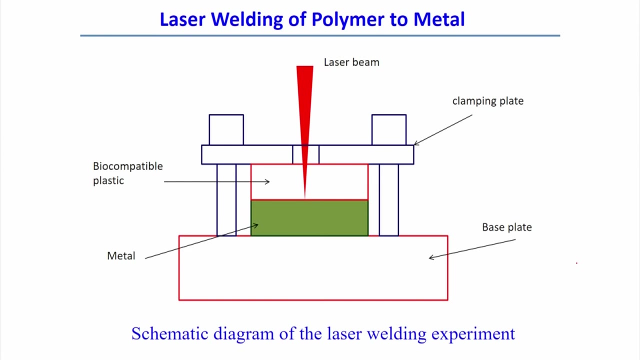 further increase in the thermal input causes a decrease in the strength. So therefore some optimum amount of the thermal input is required to get a good joint between the metal and the plastic. So here you can see that joining schematic diagram in the laser welding. 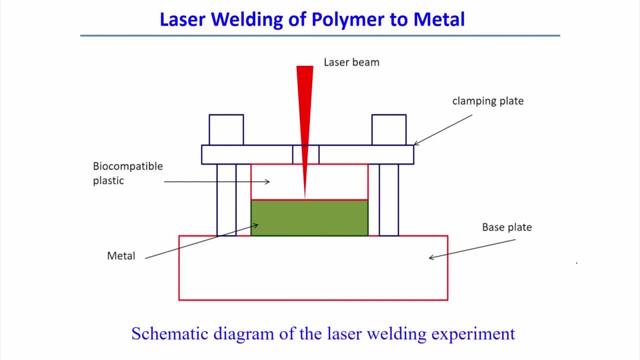 experiment, that is, the welding between the polymer to metal. it is a similar configuration to the laser transmission welding. Here you can see the, which is bi-compatible plastic. normally we can put in the upper side and in the lower side it is a bi-compatible plastic and the lower side is the metal, such that laser beam process through the transparent. 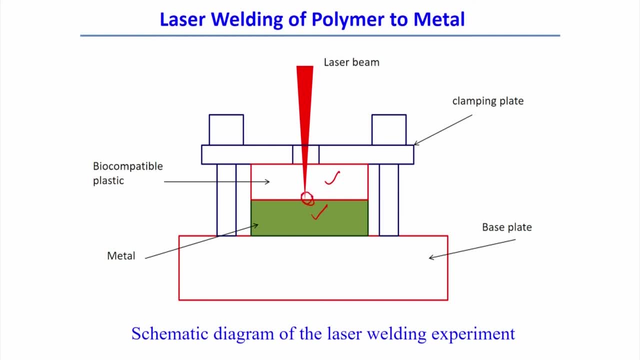 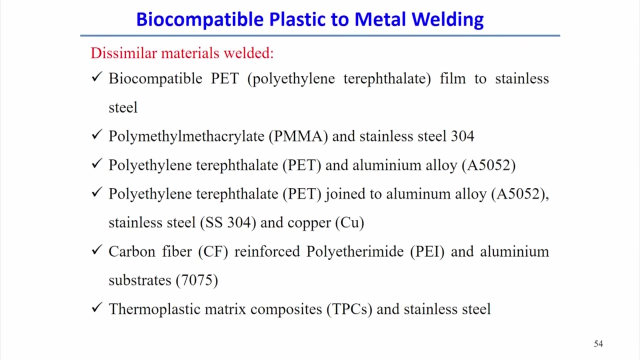 bi-compatible plastic and heat is generally released at the interface And this is the damping plate to keep on sufficient pressure between these 2 contact surface and that actually, after cooling, then finally join, weld, join is formed at the interface. This dissimilar material. there is a. there are several combination of the material. normally 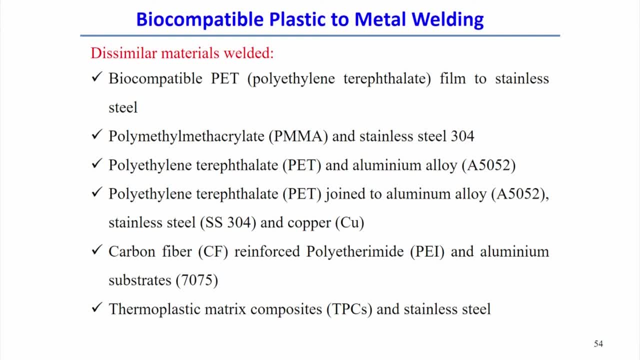 we can found out in the literature that the bi-compatible plastic to the metal- here you can see that P E T film to the stainless steel, There are several combinations of the materials in the artificial material- and the bi-compatible plastic to the material- here we can see that. 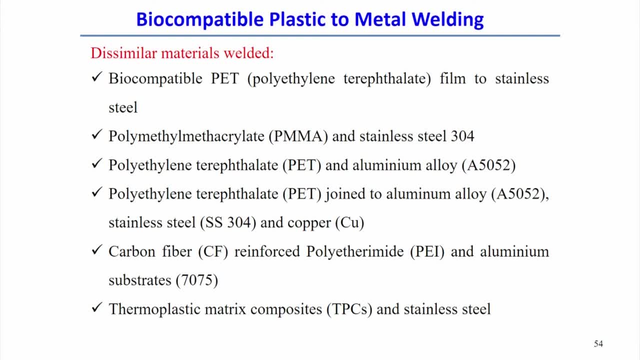 steel can be joined using this material, using this process. Then PMMA and stainless steel, 304, PET and aluminum alloy. PET and different grade of aluminum alloy, stainless steel, as well as copper, can be joined using this process. Carbon fiber, reinforced PEI and aluminum substrates can also be joined, Then thermoplastic matrix, composites, TPC and. 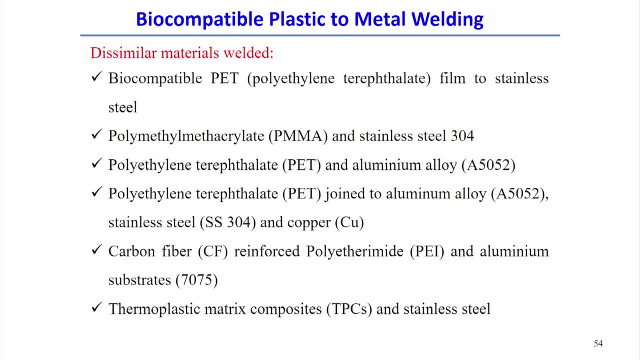 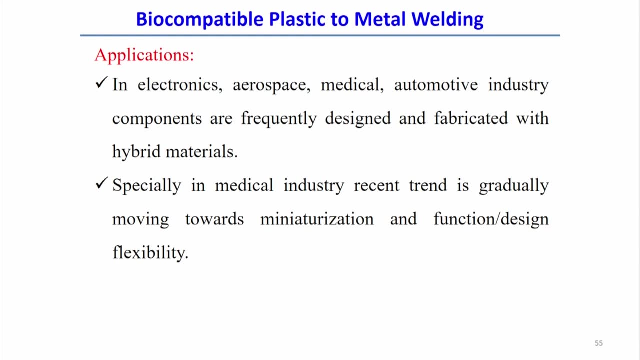 stainless steel can also be joined using this process. So therefore we can find out there is a several combination of the polymeric material and the metallic material and the joined by the in the mode of the laser transmission welding. So we can find out the typical application of the, this bi-compatible plastic, to the metal. 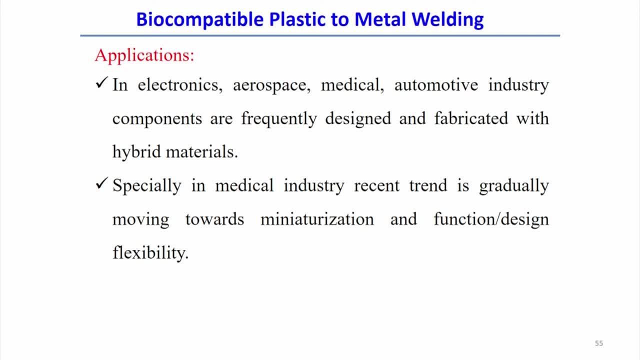 in electronics industry, aerospace industry, medical, automotive industry and therefore industry where there is a requirement Of the. particularly there is a some components of the hybrid material fabricated with the hybrid material. So in that case this process is mostly suitable. but most specifically, 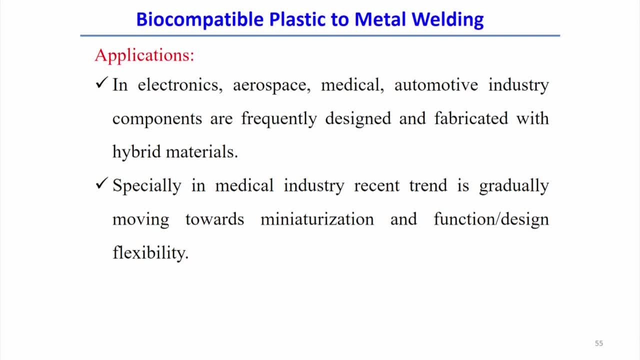 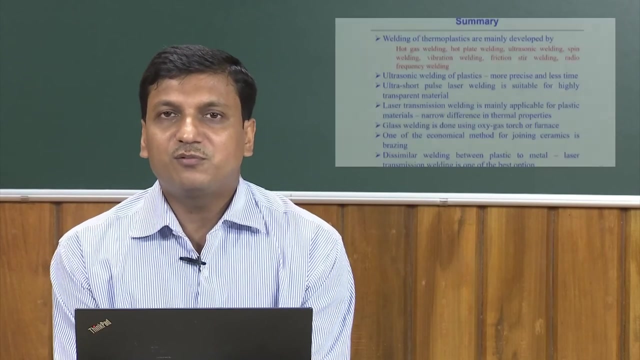 the laser transmission welding we can find out the medical industry. that is a recent trend, then gradually moving, because with the miniaturation of the components in the medical industry, So there is a increased use of this laser transmission welding in case of medical. So now up with this, all this different of the, although we have covered very few specific 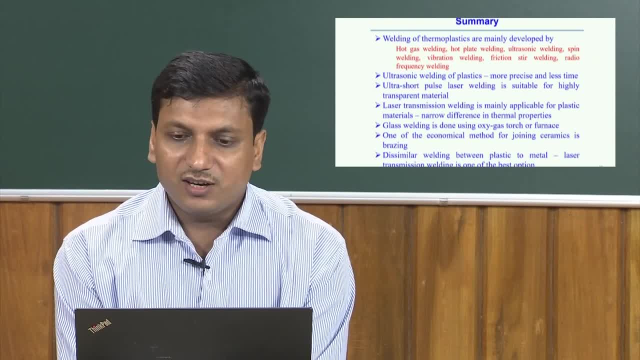 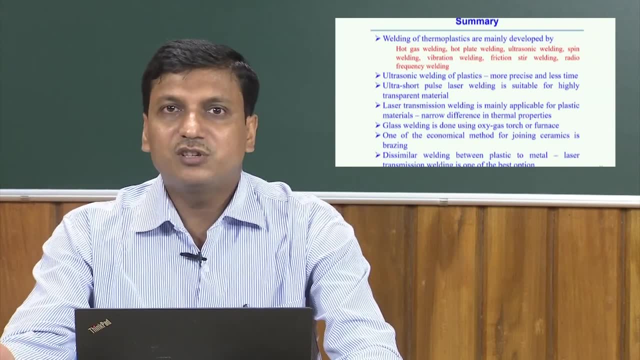 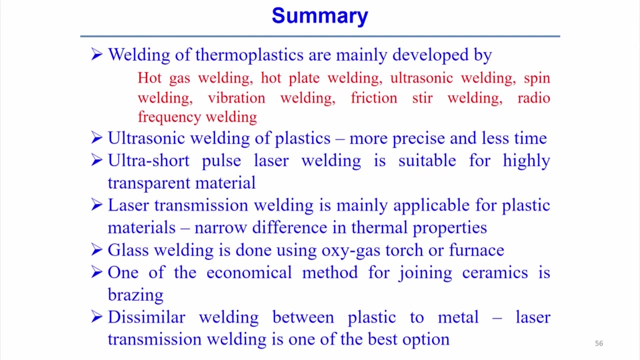 welding or joining techniques for the nonmetals and if we summarize the for the different joining techniques or some issues in the welding and joining for the different nonmetals, we can find out that the very first we discussed that welding of the thermoplastics and that 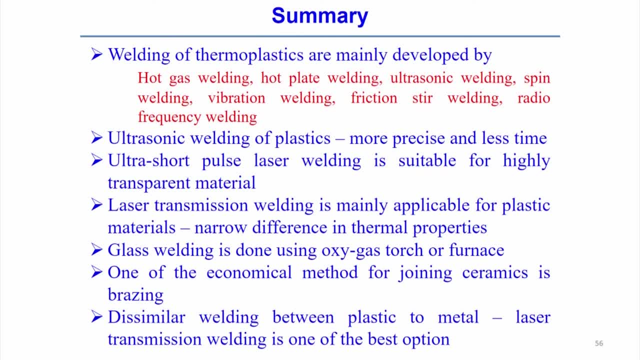 is mainly devolved by the hot gas welding, Hot plate welding, ultrasonic welding, spin welding, vibration welding, friction state welding and frequency radio frequency welding. these are the typical method methodology followed for the welding of the thermal plastic material. but among those methods, welding techniques. 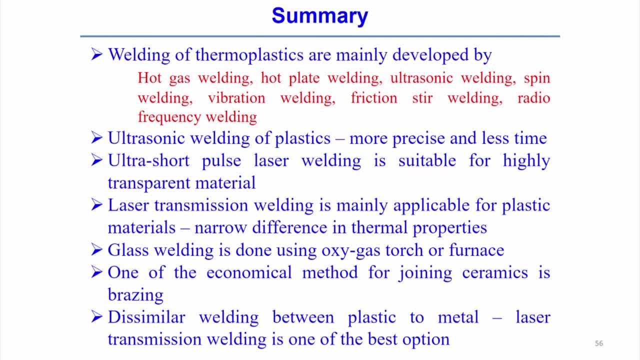 the ultrasonic welding of the plastics, that is, the, in this case more precisely, control. that is very small zone and very thin plate generally required and the weld cycle time is very less in case ultrasonic welding, welding of the plastics. Now, after that we discuss the ultrasonic welding. sorry, ultra. 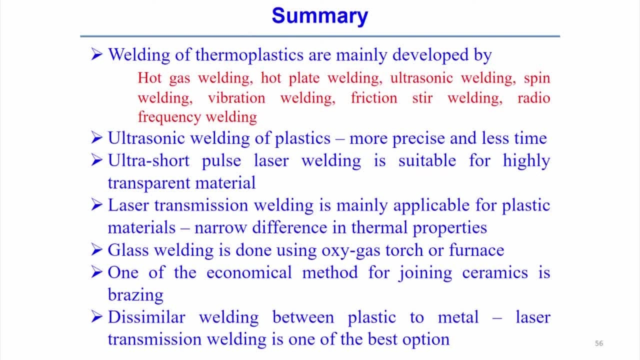 short pulse laser welding and that ultra short pulse laser welding is very much suitable for the highly transparent material, Because if that transparent material, we normally, if we transparent material, we do not use any kind of conventional laser welding process. and in this case, if you use the ultra short pulse laser, So that ultra short pulse 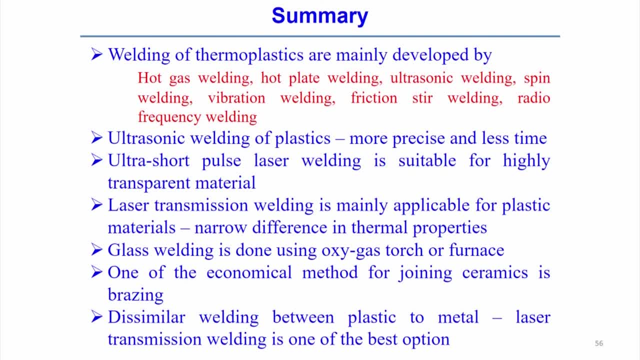 laser, when it is passes through the transparent material, So there may be the possibility of the absorption of the laser energy at this point, and specifically this happens in case of the ultra short pulse laser. So that is the one typical points to be remember when 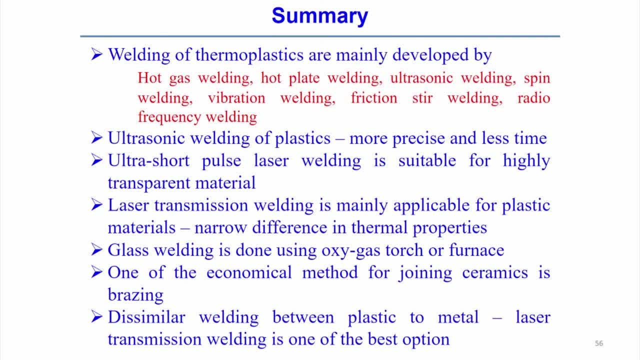 case of the application of the ultra short pulse laser. but of course there is a alternate of using the ultra short pulse laser that is called laser transmission welding. that is also developed And in that case also we can use the one transparent material. but if the using the specific 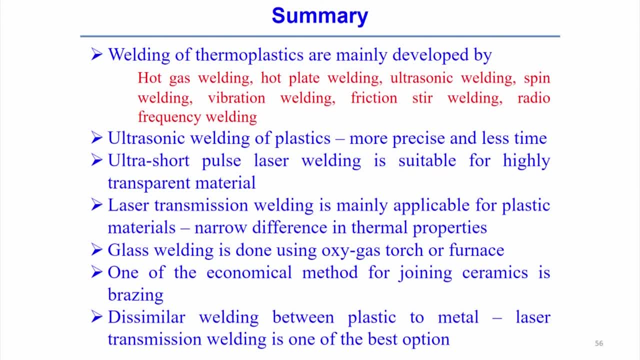 laser at the and with the certain wavelength, if that laser passes through the, both the material. So in that case some absorbing layer can be put between this two transparent material and then that absorb layers, some absorb the laser energy and that clears the amount, clears the heat in at the interface and that is responsible to join the. 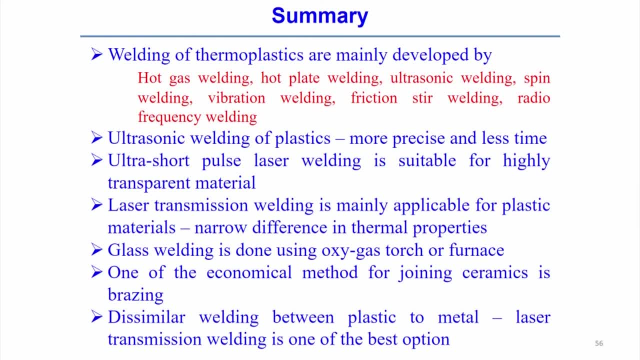 two transparent material. So in that way laser transmission welding is also developed, and using the conventional laser process Then glass welding. all the very limited welding process exist for in case of the glass welding, folding glass welding process. So here mainly we can use that oxy gas torch or furnace to 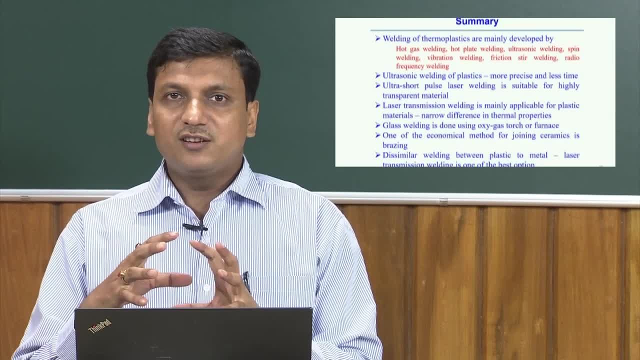 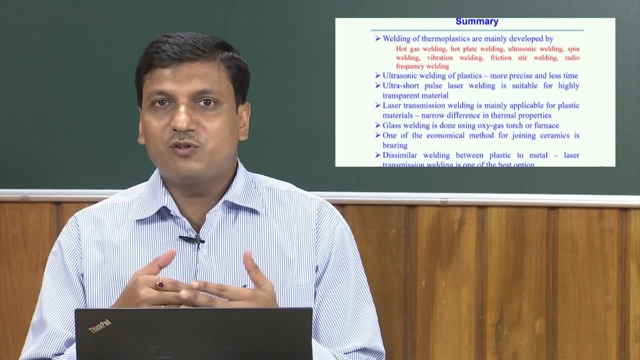 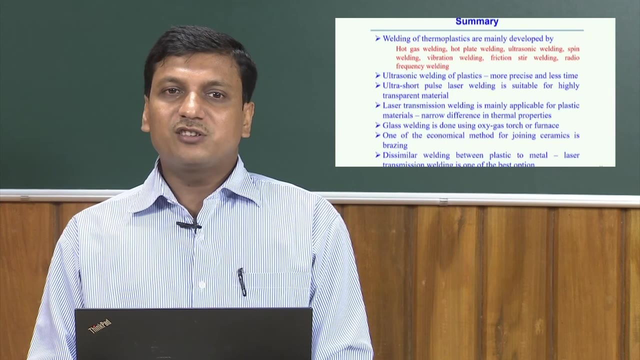 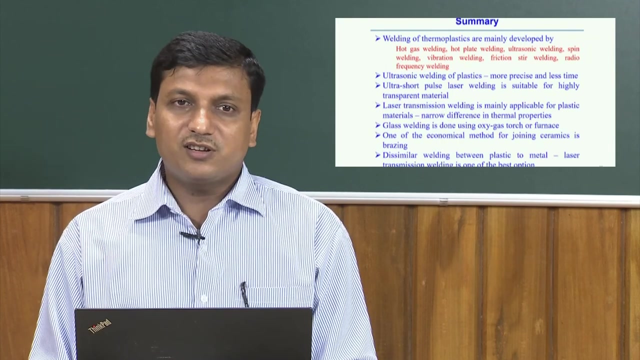 brings the flexible or may be to brings the viscous nature of the glass such that when, When they are in contact, this at this mode, when they are in contact to components, then the readily joint can be formed in case of the glass. But overall we can find out the welding of the glass. there exist very limited techniques. 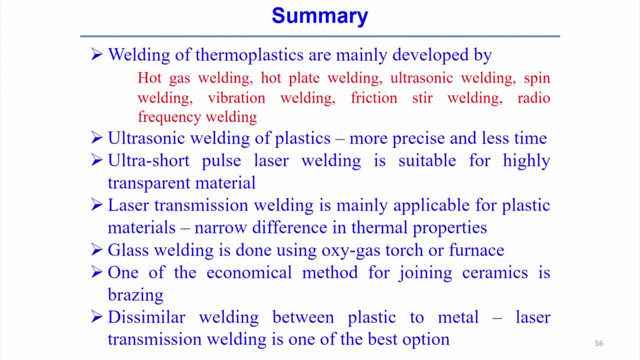 One of the most economical method for the joining ceramic is the brazing. Of course this technique having one economic brazing is the one of the economical technique, but it is having some other limitation also. Then dissimilar welding between the plastic to metal. normally we can find out most of 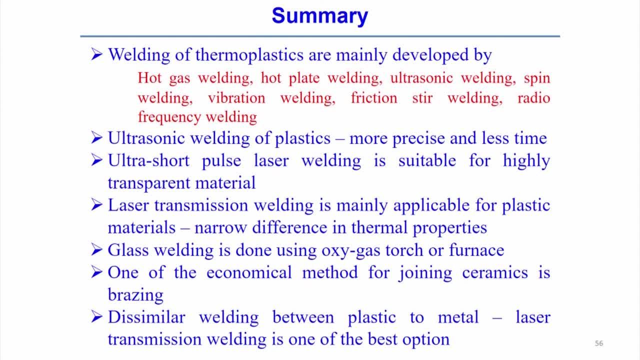 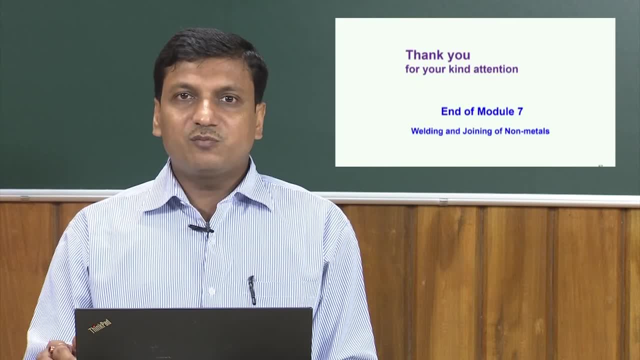 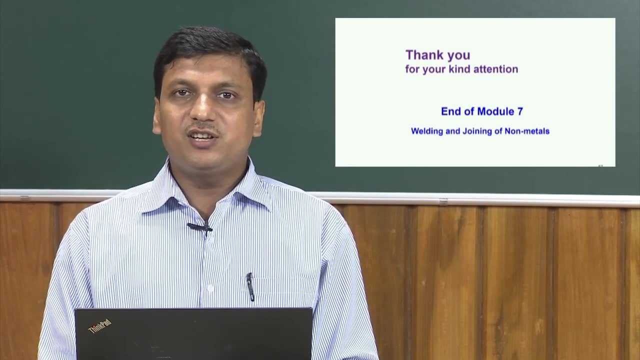 the cases we can find out. the laser transmission welding is one of the good option for the joining between the dissimilar plastic to metal. So in this module we have discussed that. different welding techniques, several issues, advantage, disadvantage. So in this module we have discussed that different welding techniques, several issues. advantage advantage: Different application area. for the welding and joining of the nonmetals, however, there is a need for extensive review of works till there is a so. many other techniques can also exist, especially for the joining of the nonmetals, But we have covered in a very few selective techniques in this case. Thank you for watching.